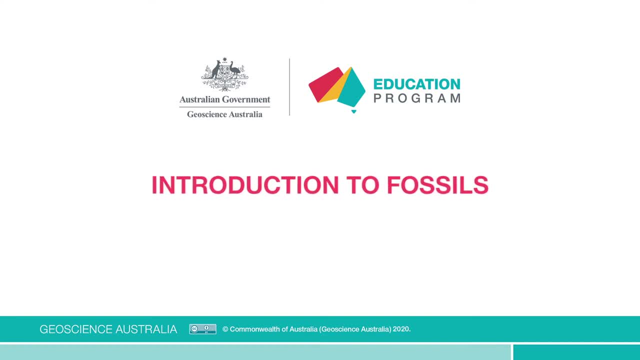 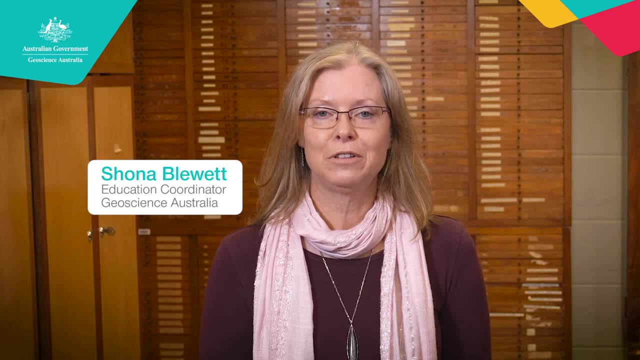 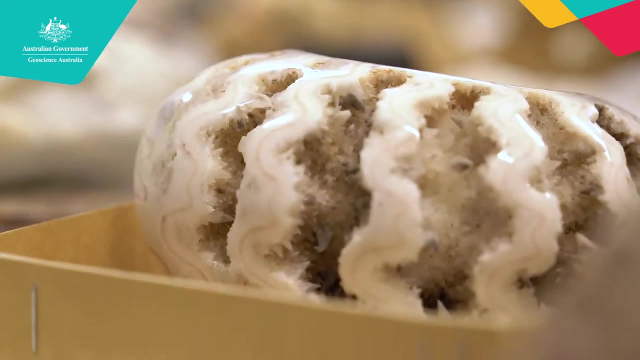 Hi, I'm Shona from Geoscience, Australia. Today we're visiting the National Mineral and Fossil Collection and we're down in a room in the basement where most of it is stored. This is a place that visitors don't normally get to see. I have Josh with me today and he's going to help us to learn. 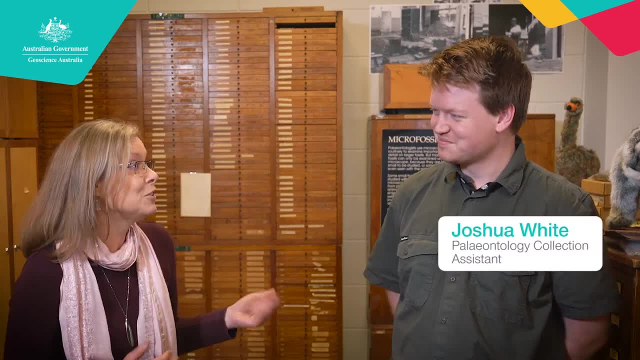 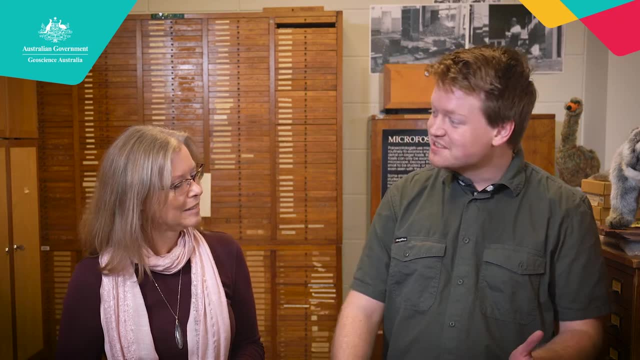 more about fossils, Josh. first of all, what is a fossil? Well, that's a great question, Shona. Fossils are the remains of ancient life forms that once existed on Earth. They can be thousands of years old to billions of years old. There are two types of fossils, usually Body fossils, such 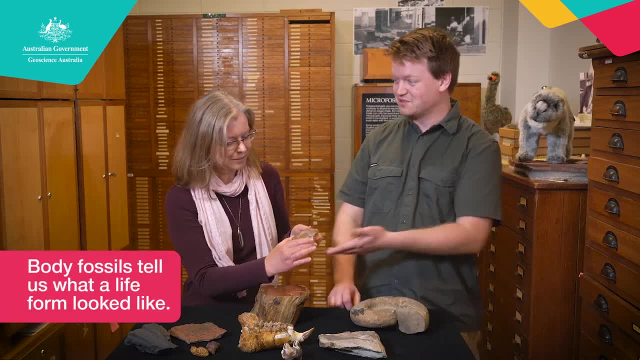 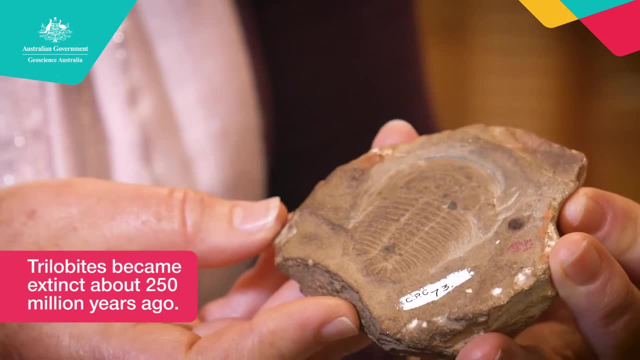 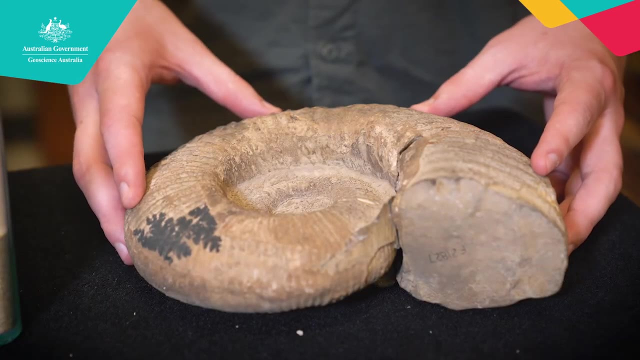 as this trilobite, which is approximately 520 million years old. And am I right in saying these used to swim around and crawl on the floor of the ocean? Yes, They didn't live on land. No, What else have we got? We've got fossilised leaves here, Ammonite, which is also a marine organism, The 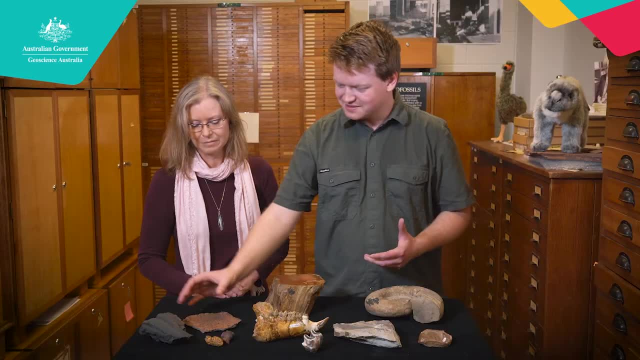 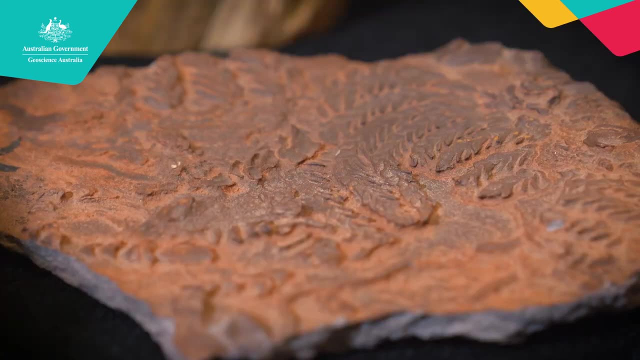 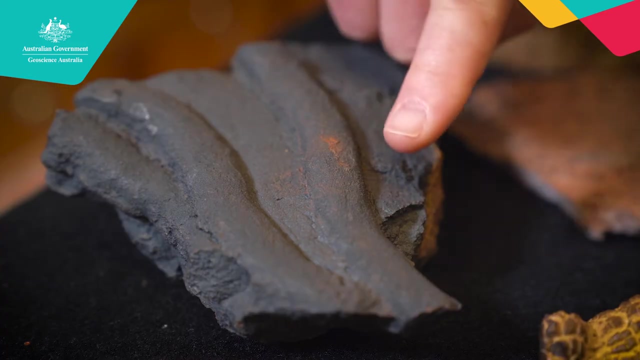 other type of fossils are called trace fossils, such as these worm burrows here or these arthropod trapways, likely made by a trilobite. So that would be a trilobite crawling along on the sand. Yes, And this would be some sort of worm eating its way through the sand and leaving a trail. 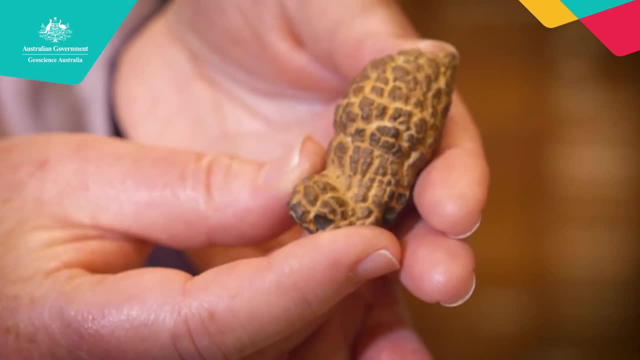 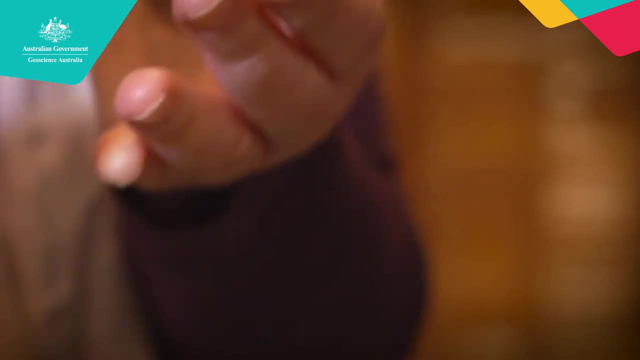 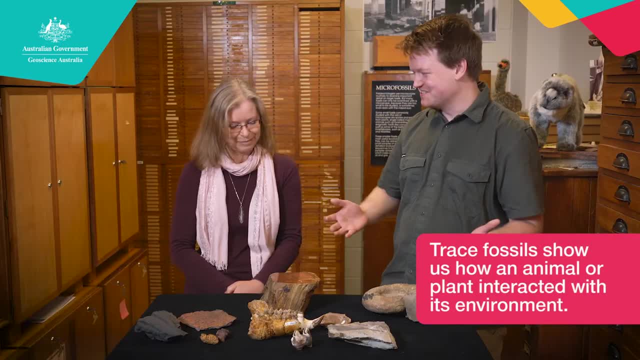 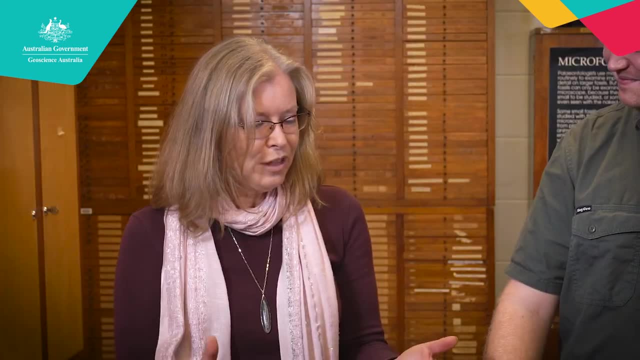 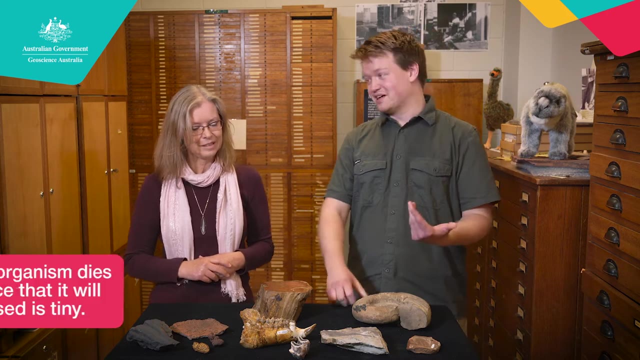 this is solid rock, Yeah, solid rock. And what trace fossils do? is that they help us infer the behaviour of the animal, Or what are they in case of fossilised poo? So these are amazing. These are beautiful specimens. How do these fossils form? Fossils are very special because they are. 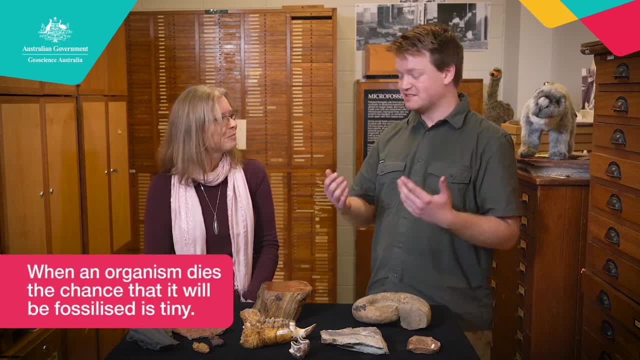 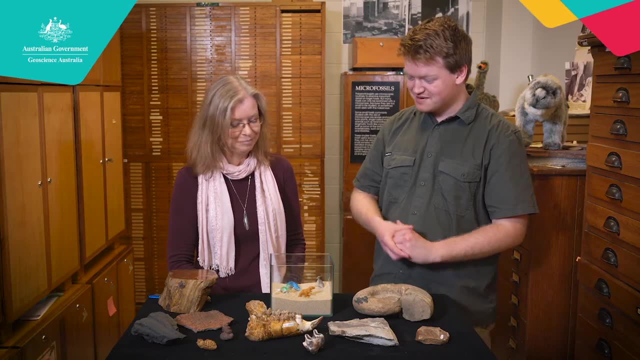 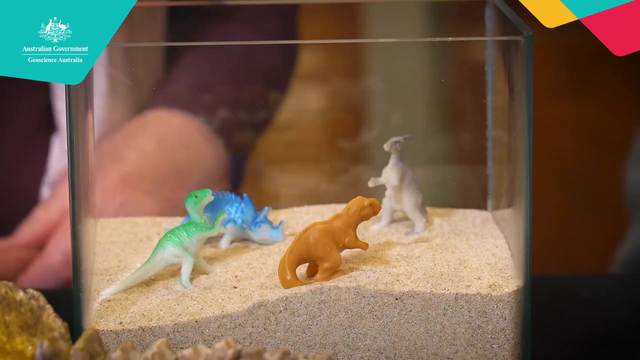 extremely rare For an animal to be fossilised. it takes a series of unique events To help show that I have this demonstration here. Imagine this as a Cretaceous riverbed about 80 million years ago And all these dinosaurs have come for a drink of water, Unfortunately for them, however. 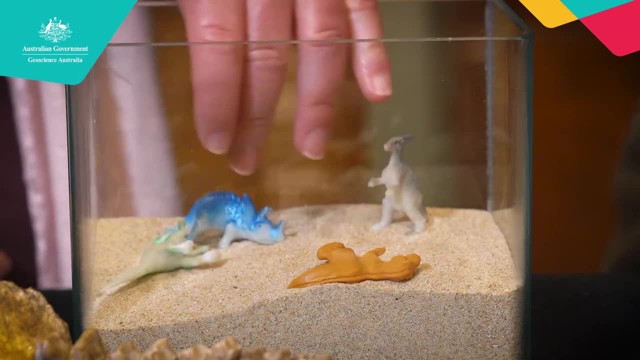 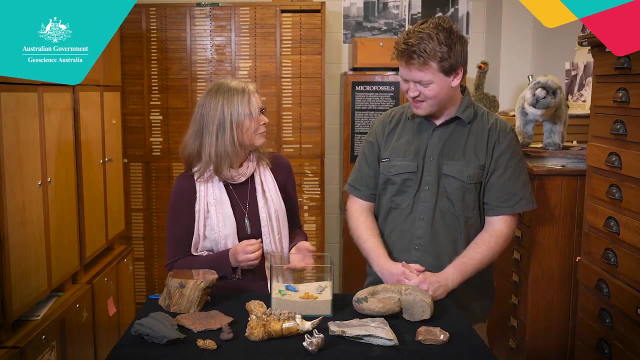 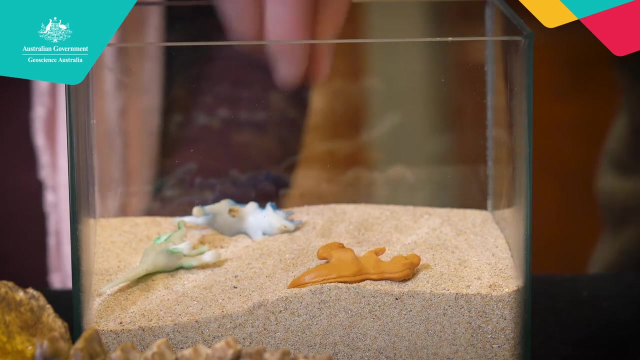 a landslide or a flash flood event occurs and kills all the dinosaurs off. Oh, poor things. We have all these dead dinosaurs. What happens to their bodies? Well, as they decay, they are eaten, scavenged off by predators. So all their bones and soft bits are taken away, disarticulated. But 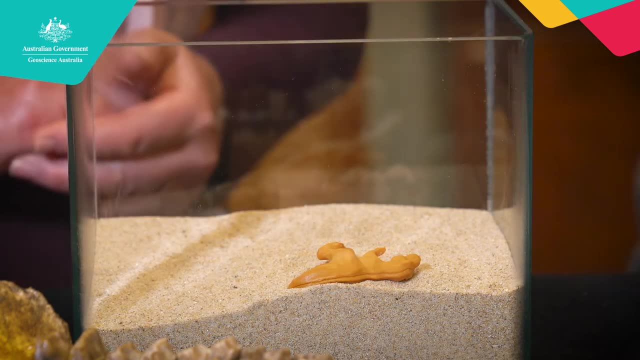 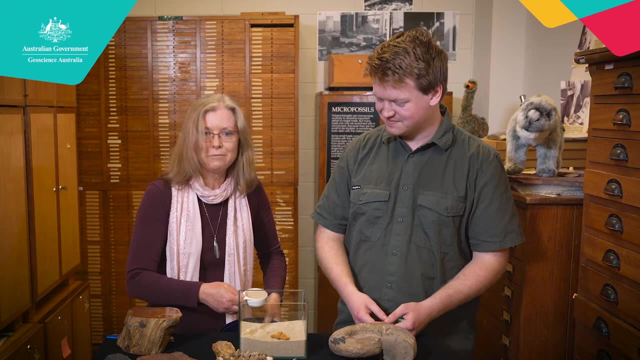 we have one left. What's going to happen to this? Fortunately for us, this little guy will be rapidly buried by five or seven of them. So imagine we have a big flood that carries a lot of sand, and that sand starts to bury our 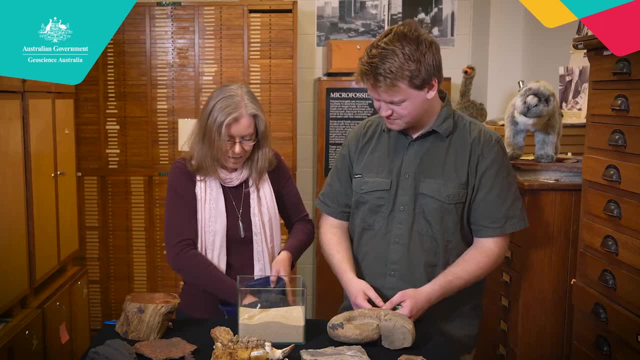 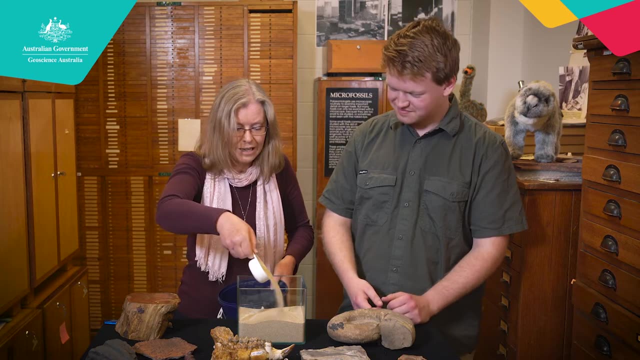 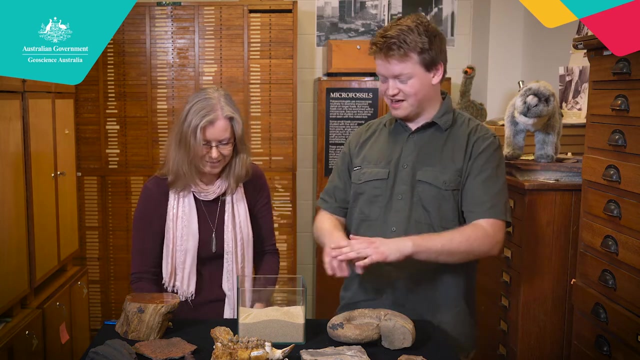 dead dinosaur- And this could happen over many, many years- building up many, many layers of sand and mud. And what's happening to our dead dinosaur down there in this time? As sediments get layered on top of the animal, it slowly compresses into the bone and replaces. 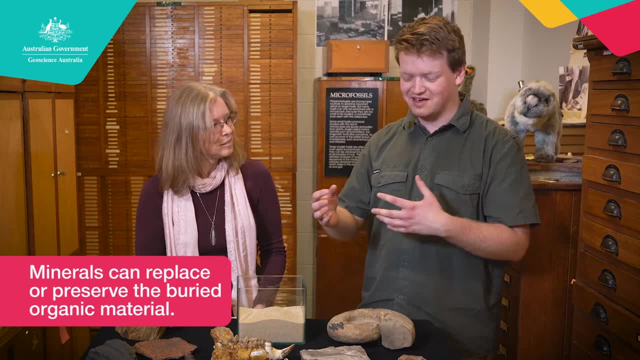 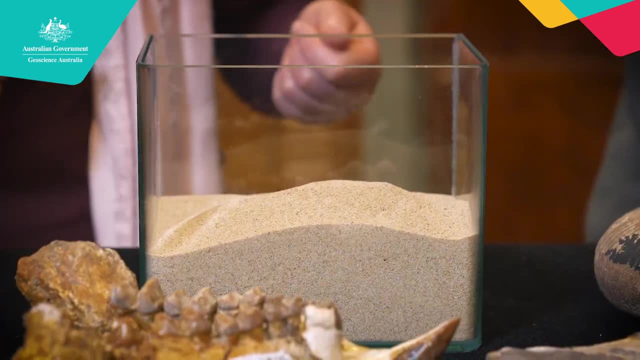 the organic material with the rock. So the animal's bones get slowly turned into stone, So it's fossilized down there. but this could be way down underground After millions more years. maybe this section of the crust is in a different situation. It could be uplifted. 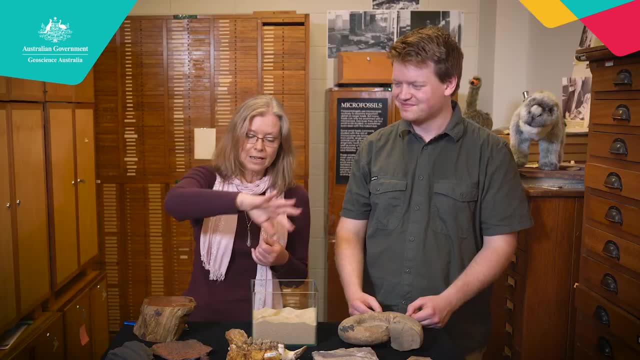 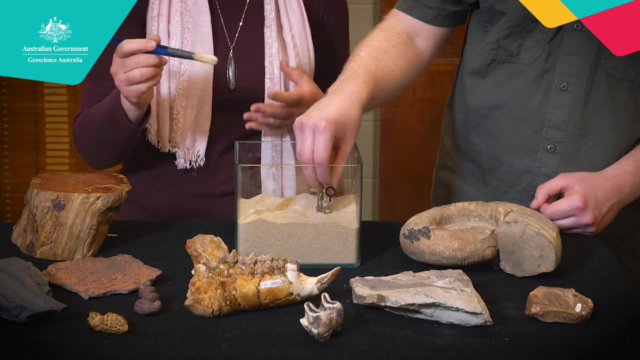 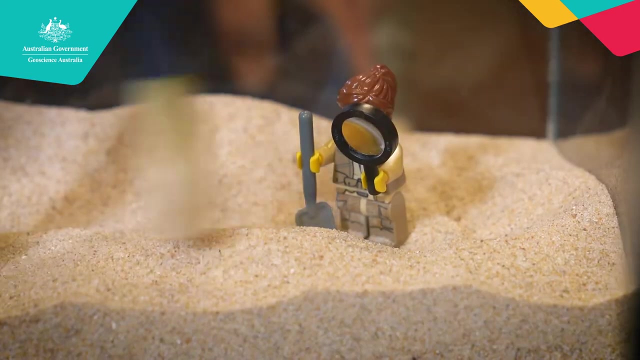 and we could have weather and erosion removing the layers of rock above And we might get to the 21st century. and we've got an explorer. a geologist or paleontologist is out exploring around and happens to see a little glimmer Of a bone in the rock and they might excavate a bit. 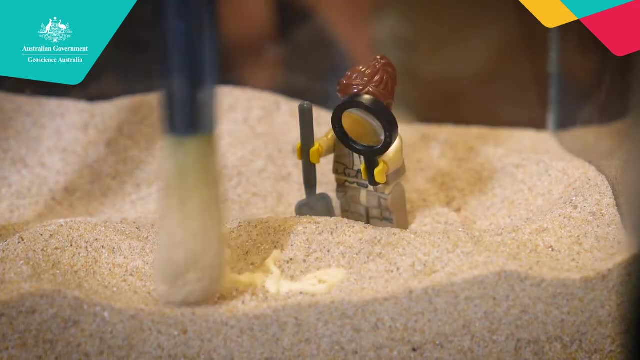 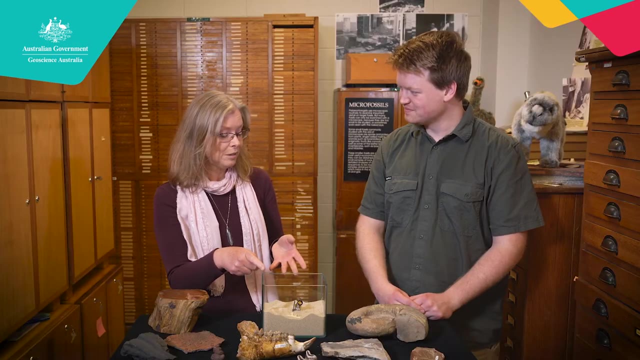 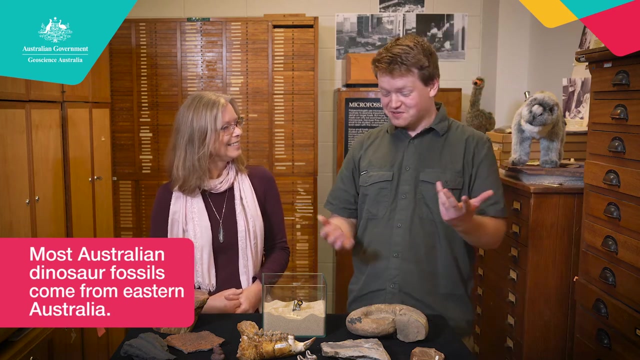 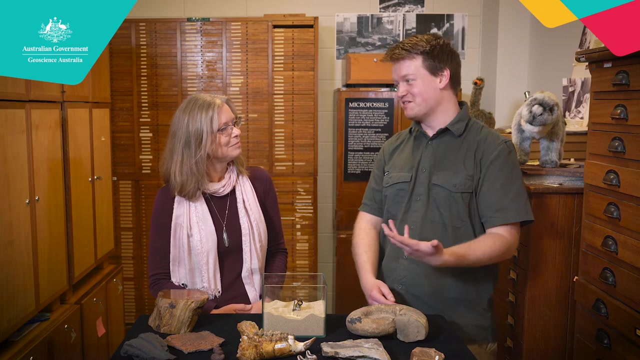 more and reveal fossilized dinosaur. Now we know how fossils have occurred. Why do scientists collect? But what use are fossils to us? Fossils are really useful for actual scientists because fossils are a gateway into the past and we can use this to help understand how Earth and life has evolved over time. 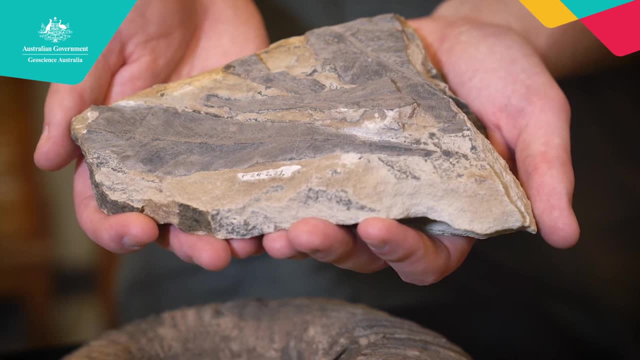 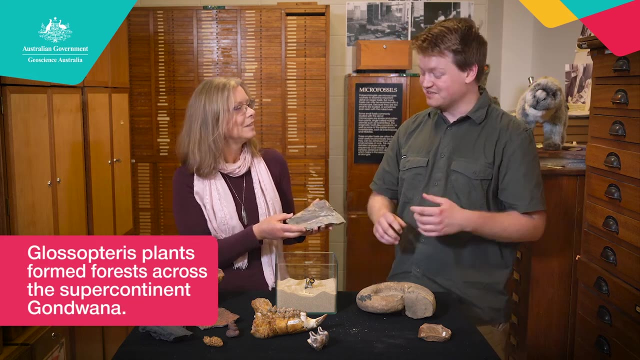 For example, this Glossopteris here is only found on southern continents such as Antarctica, Australia, South Africa, Asia and India. These show us that all these continents were joined together at one point in Earth's history. What about this?